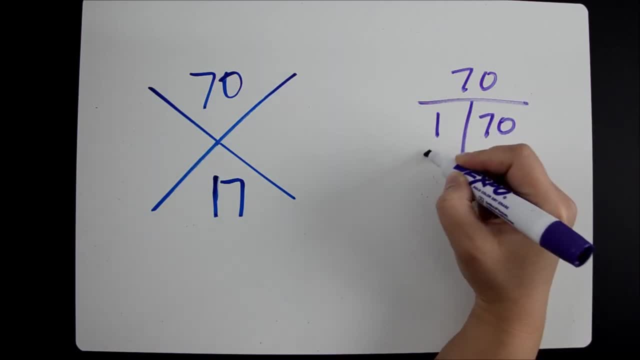 are positive, but we're going to go ahead and list out all the factors anyway. So 2 and 70,- I'm sorry, 1 and 70,- 2 and 35,, 5 and 14,, 7 and 10.. So here it's a little bit more obvious. 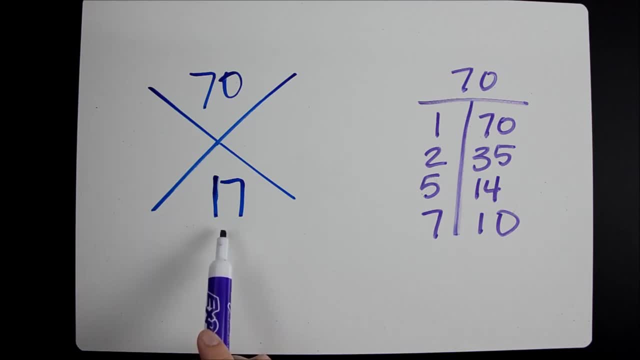 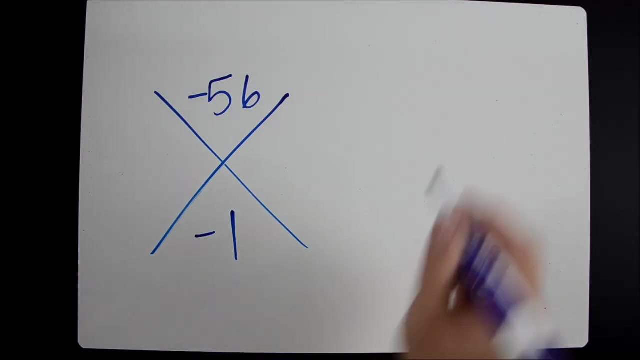 The pair that adds up to 17 in this case would be 7 and 10.. And it doesn't matter which order we put those two cells in or put those two numbers in. So let's take a look at a problem where we have a negative product, a negative sum. We're still going to create a table of factors. 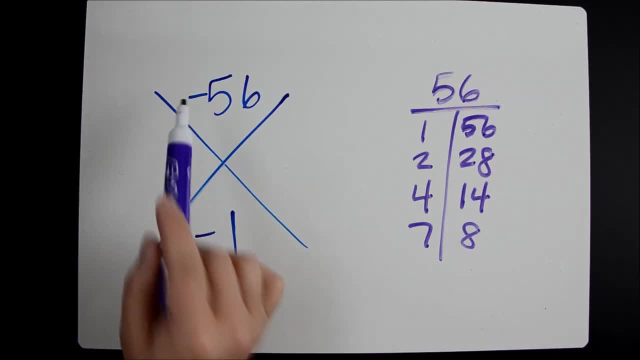 This is a little bit tricky. We know that one of the numbers is going to have to be negative in order for it to result in a negative product, And so it's pretty obvious that the pair has to be 7 and 8.. We just have to figure out which number we'll add to give us negative. 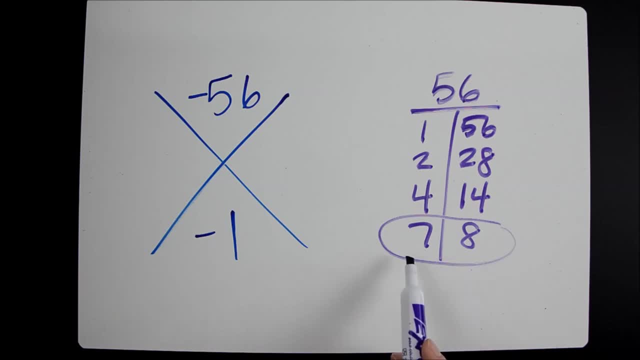 1 when we make it negative. If I make the 7 negative, negative, 7 plus 8 results in a sum of positive 1.. So that wouldn't work. What we're going to have to do is make the 8 negative, And when we add 7 and negative 8, it does give us a sum of negative 1 and 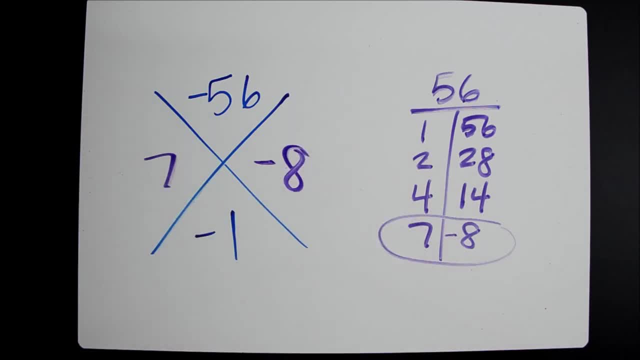 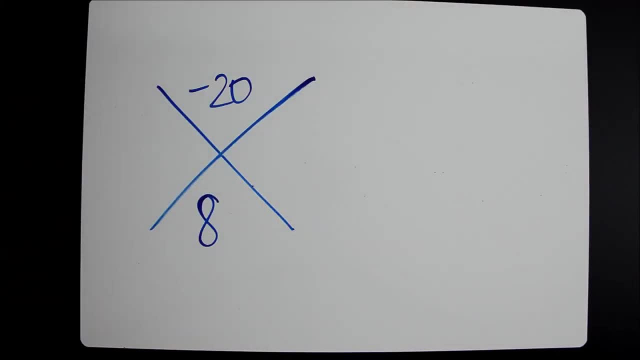 a product of negative 56.. Let's take a look at one more example. So here we need to find two numbers that multiply to give us negative 20, but we'll add to give us a positive 8.. So the factors of 20 include 1 and 20,, 2 and 10, and then 4 and 5.. So we know that one. of our numbers is negative 8.. And so we're going to add 2 and 5.. And so we're going to add 2 and 5.. And so we know that one of our numbers is negative 8.. And so we know that. 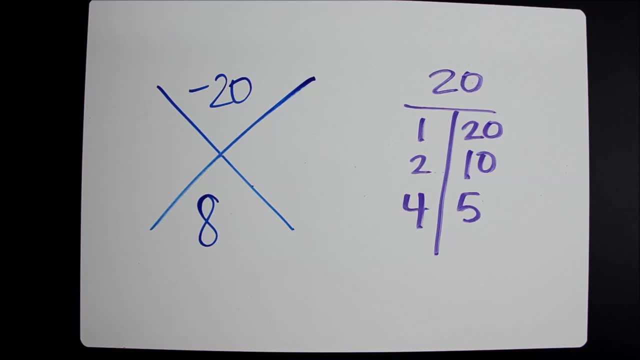 two pairs of numbers will have to be negative in order for it to result in a negative product, And the pair that makes the most sense in this case, in order for it to add up to 8, would be 2 and 10.. So if I make the 2 negative negative, 2 plus 10 does result in positive 8. And so